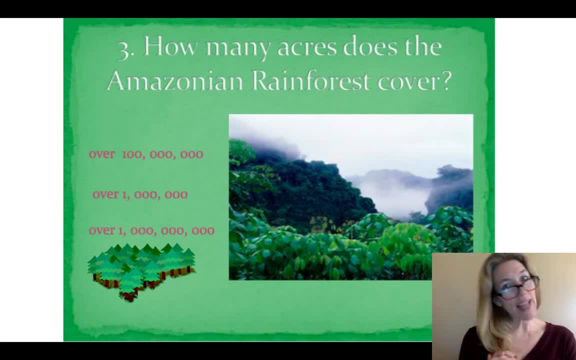 Number three: how many acres does the Amazonian rainforest cover? Okay, so let's think about that. How many acres does the Amazonian rainforest cover? Okay, so let's think about that. look at your three choices and would you believe it is the very last option? one billion acres a. 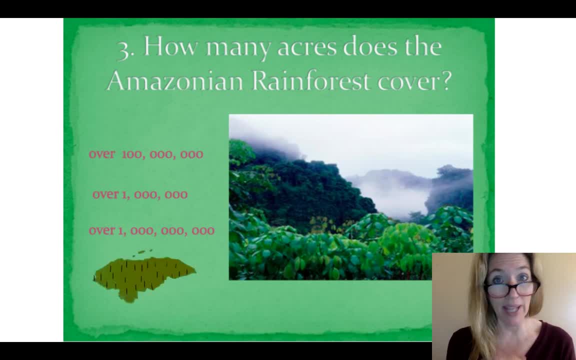 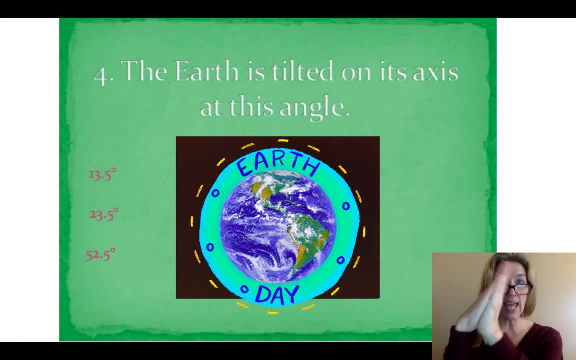 beautiful rainforest where all those wonderful animals and plants exist. number four: the earth is tilted on an axis. at what angle? so i know we haven't studied this. these are just interesting trivia about our planet, and do? it is the middle angle, 23.5 degrees. moving along now to question: 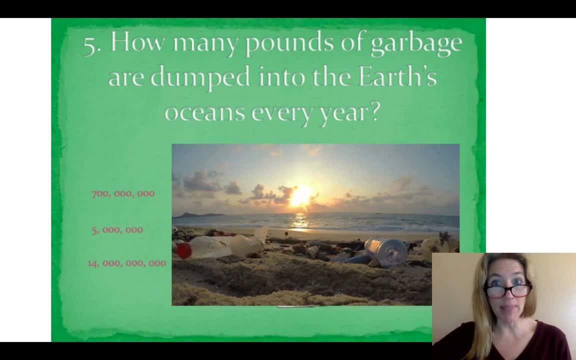 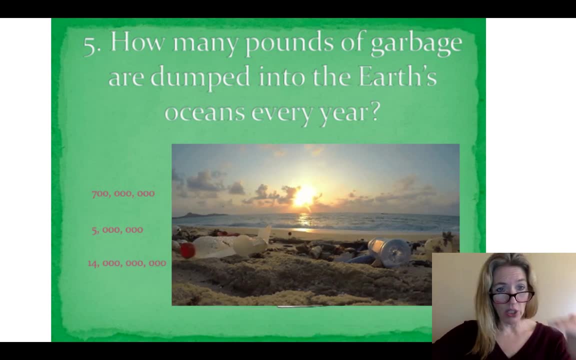 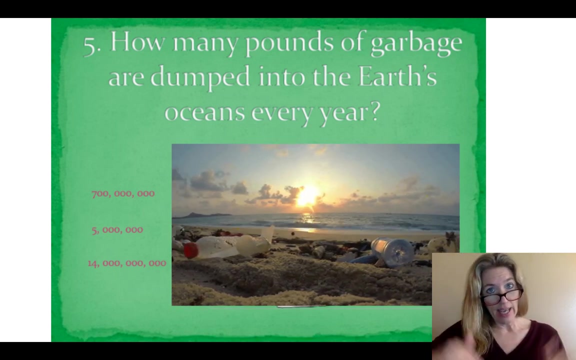 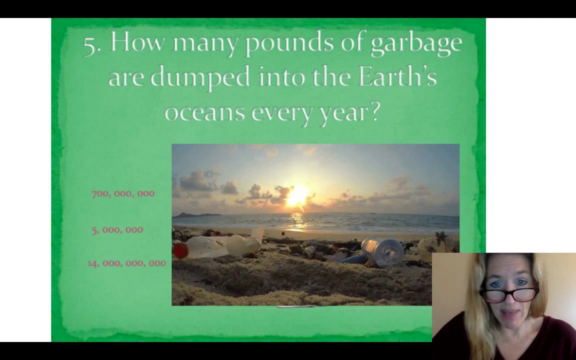 number five: how many pounds of garbage are dumped into the earth's oceans every year. this is a sad statistic, okay, so i want you to look at those three numbers and sadly i have to report it is the final answer: they're at 14 billion pounds of garbage. i found this gif and and it made me sad. 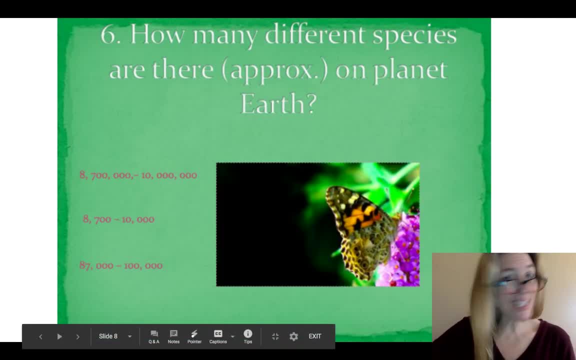 bummer, all right, number six. how many different species are there on the planet? and this is including both plants and animals? so if you look over on the left hand side, the correct answer is the top answer: eight million seven hundred thousand, all the way up to 10 million different species of beautiful plants and animals that inhabit this. 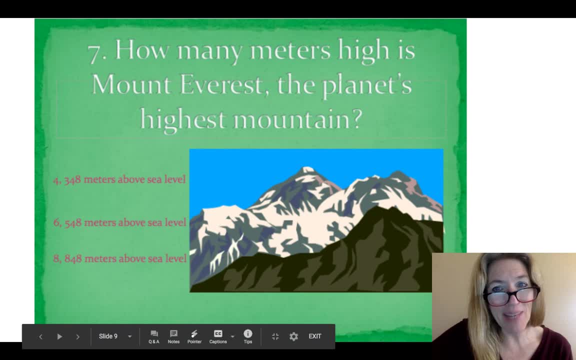 earth. okay, number seven: how many meters high is mount everest? um? i've done a lot of research on mount everest. it's in nepal and it's been on my um top 10 places to visit um for the last 10 years at least. so i haven't made it there yet, but it's very, very high. 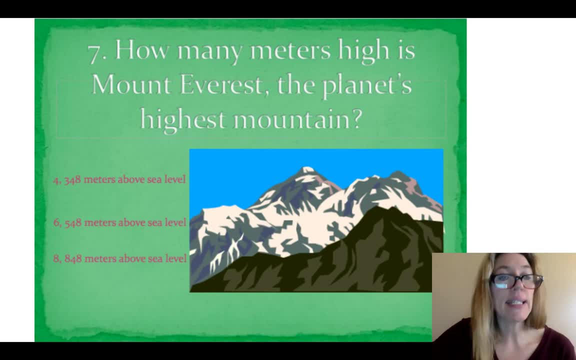 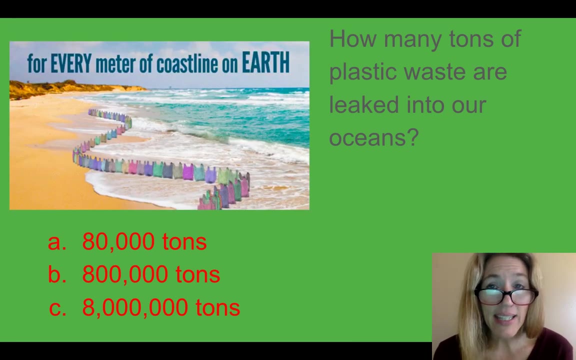 so how high is mount everest? uh, okay, it's the last one: 8 848 meters above sea level. okay, i'm moving on to number eight. how many tons of plastic are leaked into our oceans? so if you're actually looking at the gif in the top left hand corner of our screen, it actually tells you the. 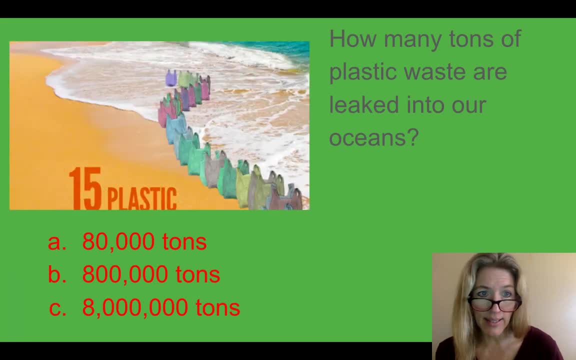 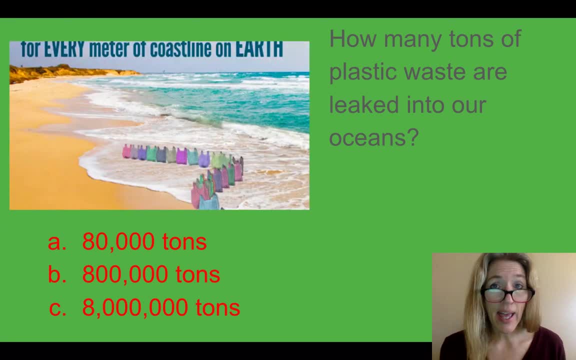 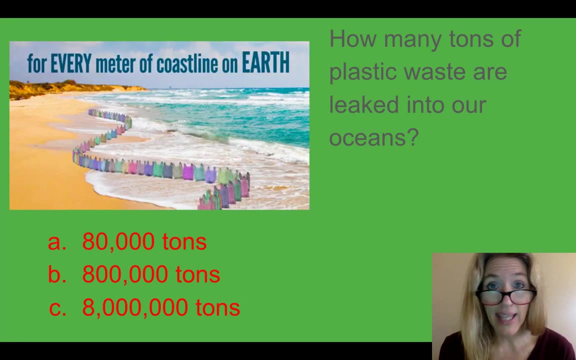 actually looking at the gif in the top left hand corner of our screen, it actually tells you the correct answer, which is eight million tons of plastic that are leaked into our oceans. so, if you're, by using glass, using a, choosing not to use plastic and reducing, reducing, 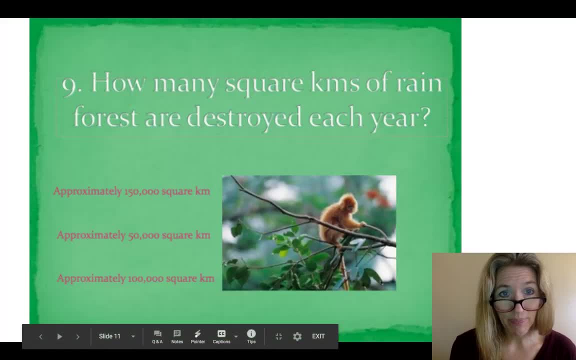 reducing the amount that we use plastic? okay, number nine: how many square kilometers of rainforests are destroyed every year? okay, yet another sad statistic, and unfortunately it's the top one. a hundred and fifty thousand square kilometers- kilometers are huge folks, and that is what is being destroyed in. 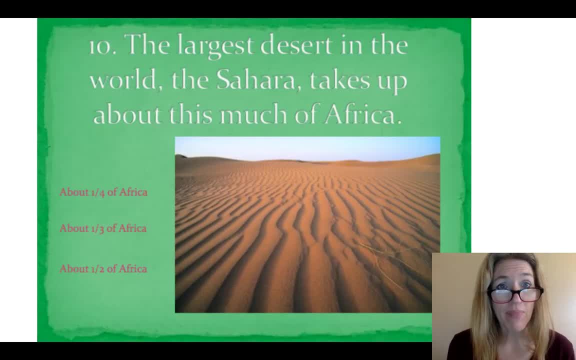 our beautiful rainforests every year. number ten: I found a question about the Sahara Desert. my husband and I actually spent some time there and my husband used to be there as a Marine and was stationed in the Sahara Desert and it's gorgeous and beautiful and, would you believe, out of these three fractions of 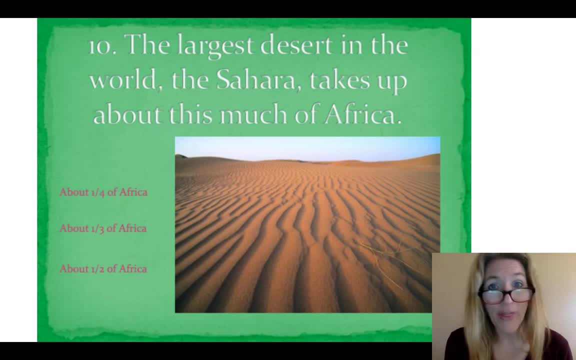 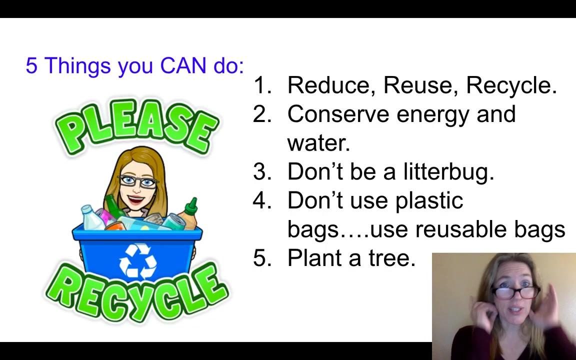 the Sahara Desert actually is one-third of the whole continent, Wow. so we have to protect these beautiful resources and lovely places on our earth. we have such a beautiful home on this planet. so you may be asking yourself: what can I do as a junior high student to to help our planet? and, as we mentioned on the 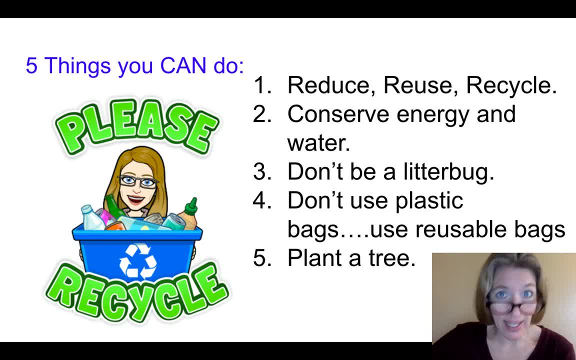 plastic slide. you know plastics are not fantastic. plastics are not fantastic. please reduce their use anytime you have a choice. I even have switched from plastic toothbrushes to bamboo toothbrushes. so every choice you make, and if you just have that in the back of your mind that you're not going to use,